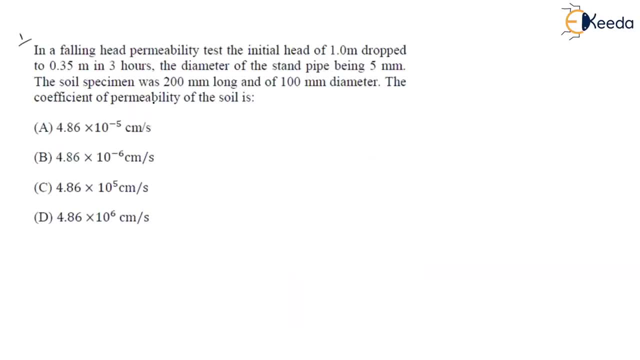 Okay, let us understand the given question. In a falling head permeability test, the initial head of 1 meter dropped to 0.35 meters in 3 hours. Okay, and in the given question itself they have mentioned that it is a falling head test. 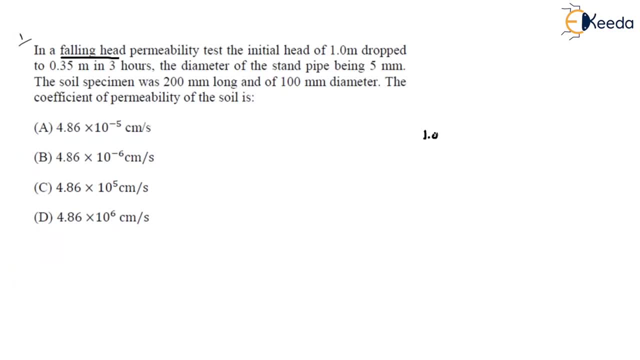 And what they are saying. Initially, if it is of head, it is 0.35 meters. At 1 meter it is dropped to 0.35 meters. In how much time? In the 3 hours time? Okay, the diameter of the standpipe. 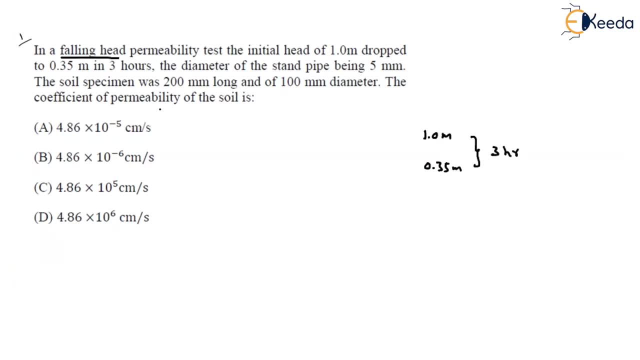 And also they are given the details of the specimen. Okay, they are asking the permeability. Oh, I think it is a direct question, isn't it? What is the formula for finding permeability for the falling head test K? that will be equal to A into L divided by. 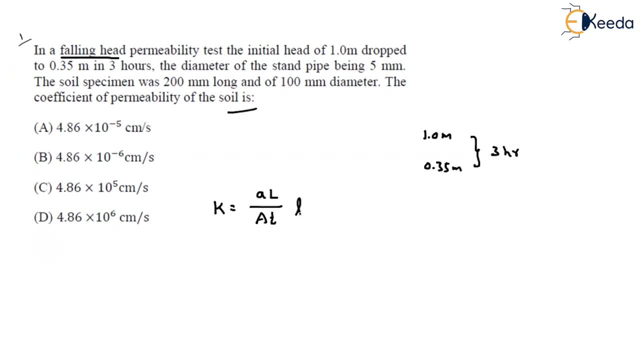 capital K, Capital A into T. Here I am writing Ln. Ln means log with respect to E, Ln of h1 divided by h2.. So what does it mean by A Small a? Small a is nothing but the area of the standpipe. 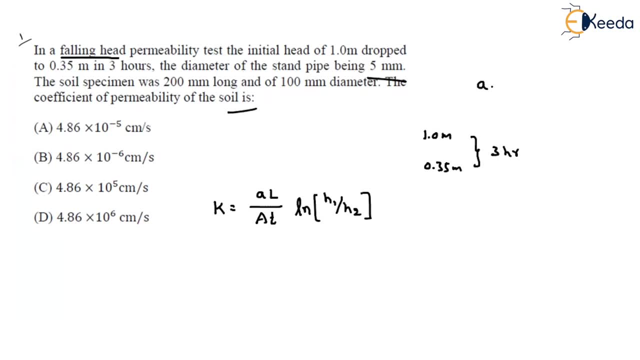 So here he said that it is a diameter. So whatever the area Area, I can write it down as a pi by 4 into 5 square. So that will be equal to pi by 4 into 5 square. 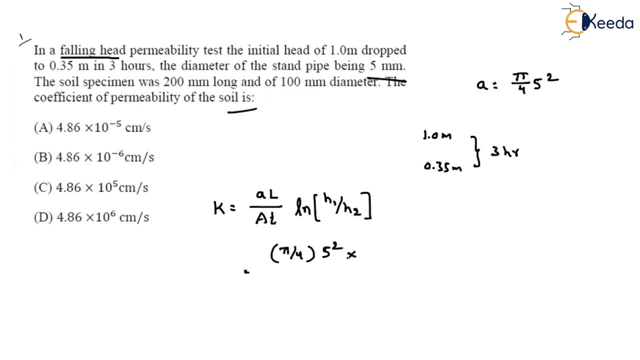 So here I am taking dimensions in mm. So let me continue with that. L is nothing but the length of the soil specimen. What is the length of the soil specimen? 200 mm. This also I am taking in mm. 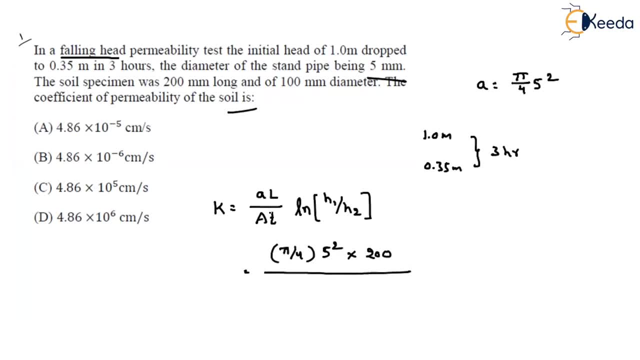 Divided by capital A. Capital A is nothing but a cross-sectional area of the soil specimen. Soil specimen is having 100 mm diameter. Then, whatever the area, again the same thing: Pi by 4. into here also I am taking mm. 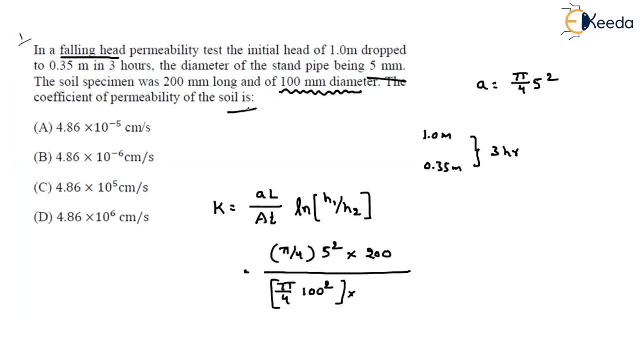 100 square. Into what? Into the soil specimen. So what is the time Time required for falling head? from 1 to 0.35.. How much it will be Here? the time is given as 3 hours And if you see the options, the options we are getting in seconds. 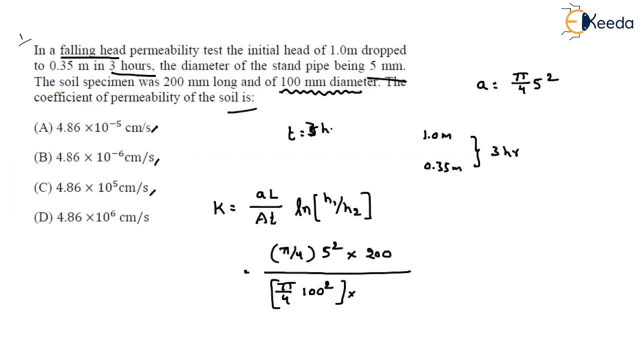 So the time is nothing but 3 hours. Then how can I convert into seconds? If I convert this into minutes, 3 into 60 minutes? Again, if I convert into seconds, 3 into 60, into 60.. 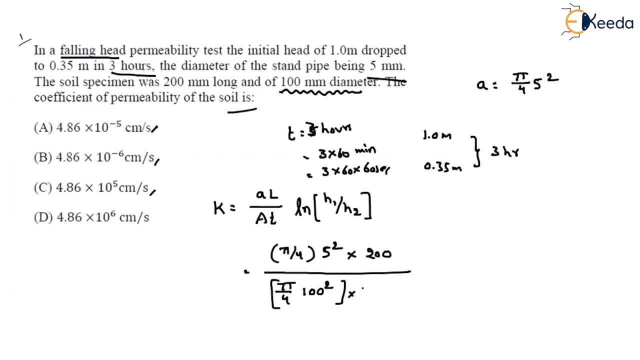 60 seconds. So what about the time? here, The time is nothing but 3 into 60, converting into minutes into 60, converting into seconds, ln. so I am writing a log with respect to e or ln. What is h1?? 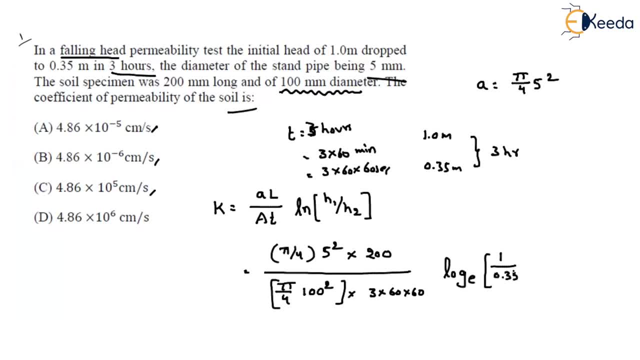 1 divided by h2 is nothing but a 0.35.. So here time we are considering in seconds And our areas and lengths we have considered in mm. So whatever the answer we will get, that answer will be in the second. 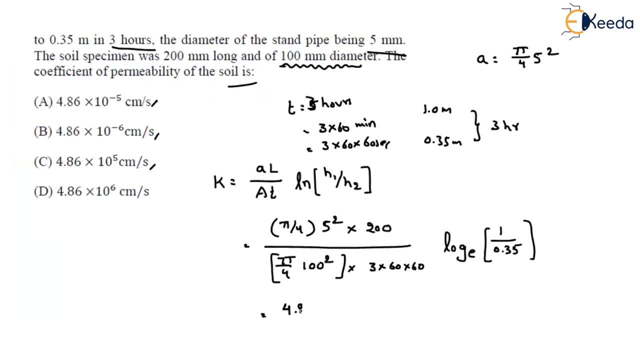 So the answer is nothing but a 4.86 into 10 to the power of minus 5 mm per second. So what is the correct option? a No. Why? Because here the unit is mm per second. So what you will do in the exam hall, you know. 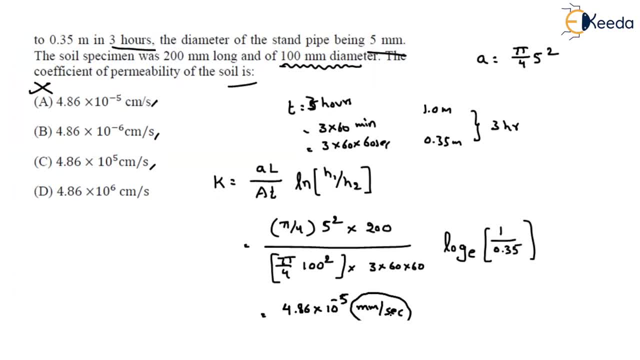 you are so very happy that very small questions came and you got the answer And without seeing these units, what you will pick it up a. But always remember while selecting the answer: please cross it with the units. Most of the mistakes the students will commonly do is with the units only. 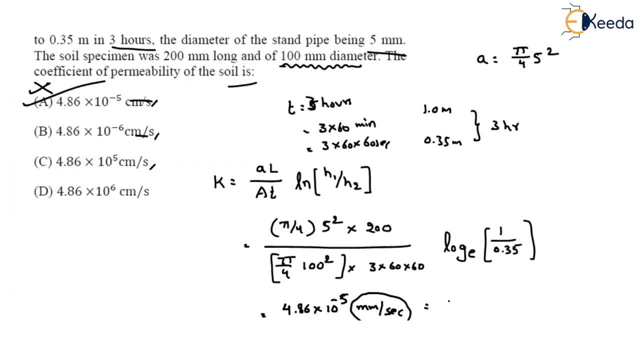 So convert this into centimeter. So if I convert this into centimeter, then the answer will be 1 mm, equal to 10, to the power of minus 1 centimeter. So minus 1 we will add here. So what will be the option? 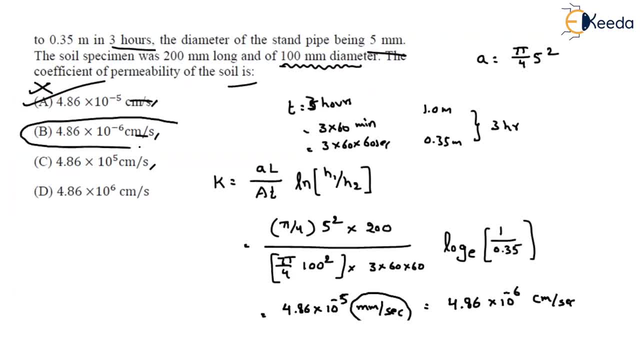 4.86 into 10, to the power of minus 6 centimeters per second. So this is what the correct option. So this is a direct or far-novel unit problem. Just you have to substitute in the proper units. 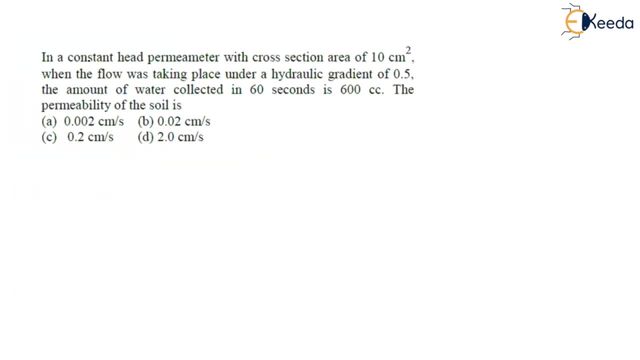 That's it Next. So what is the given question In a constant head permeameter- so this is also nothing but a test Permeameter- is equipment used to find the permeability of a swell specimen In a constant head. they have given what is the cross-sectional area. 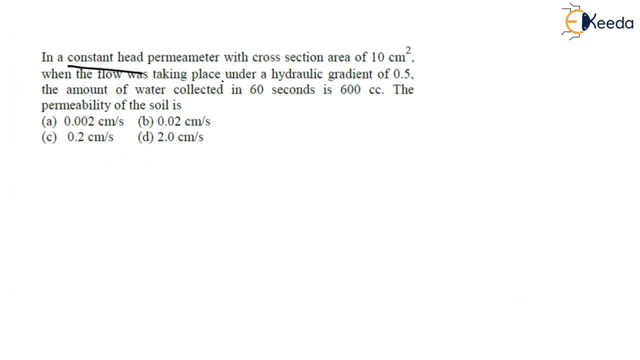 10 centimeters square When the flow takes place. the flow is taken place under a hydraulic gradient of 0.5.. The amount of water collected in 60 seconds is 600.. So, first, what they are asking. They are asking us to find out the permeability. 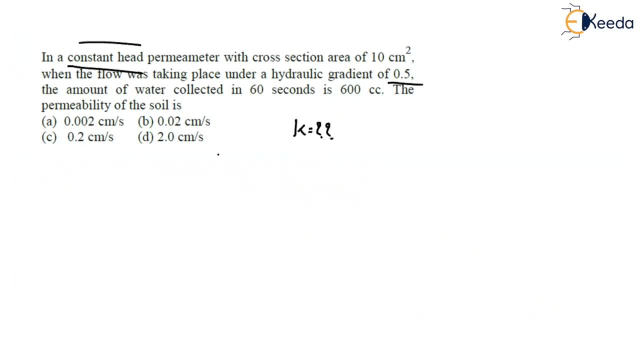 For finding permeability in a constant head test. what is the formula we can use? We can use Q equal to K, into I, into A. What is the Q Discharge through the soil? So here, amount of water collected. So what about the discharge then? 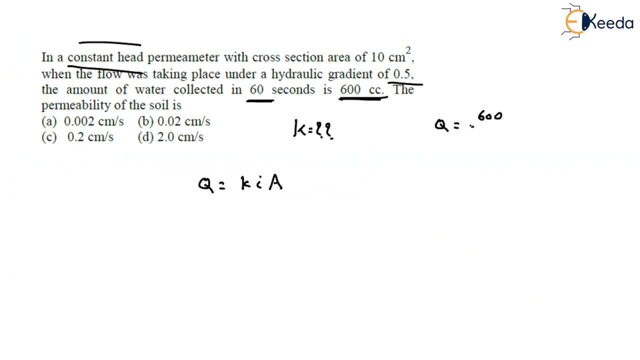 Q equal to what is the volume of water collected? 600 cc, 600 centimeter cube. In how many seconds? 60 seconds. So if I solve this, how much? I'll get? 10 centimeter cube per second. 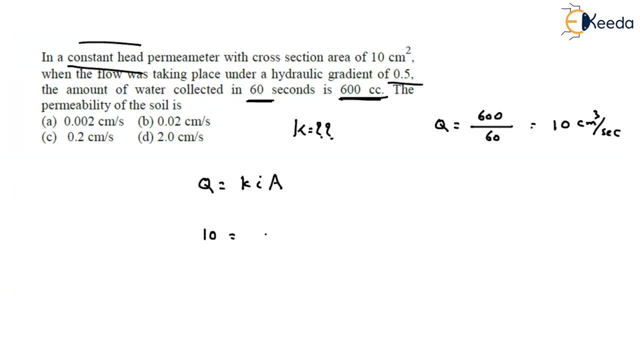 Right, So here I'm taking 10.. That will be equal to K. into what about the I value Hydraulic gradient? it is directly given. 0.5 into A is nothing but a cross-sectional area. How much it is given. 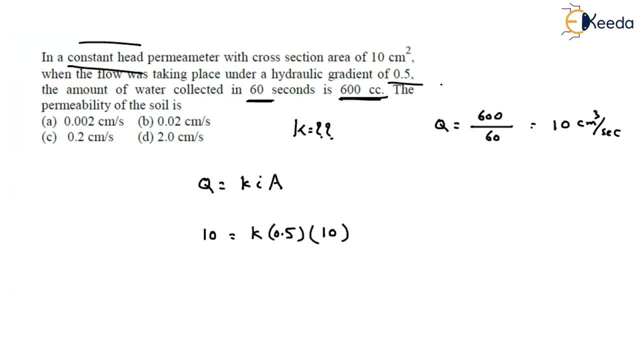 10 centimeter square. If you see the units here directly, they are given every unit in centimeters and second. So there is no need to conversion here. So that implies what is the K value: 2, 10 by 5, 2.. 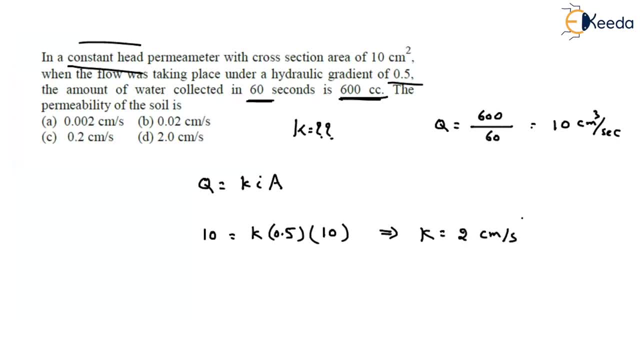 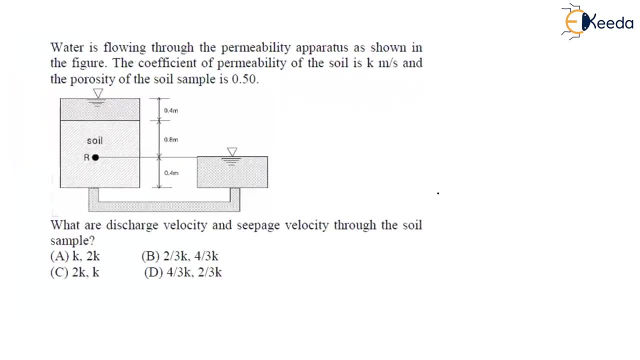 So K value is nothing but 2 centimeters per second. So these are nothing but just formula-oriented questions, isn't it? And see the next question. Water is flowing through the permeability, The permeability operators as shown in the figure. okay, 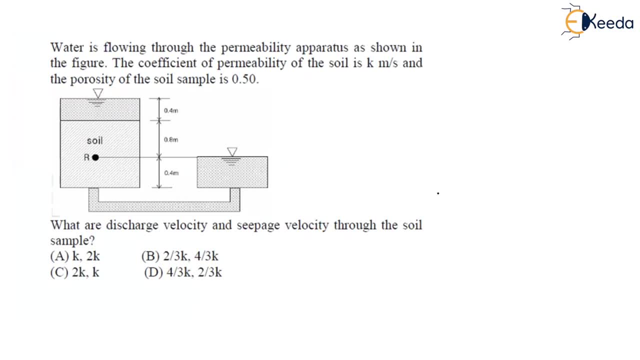 There is some flow arrangement here. The coefficient of permeability of the soil is K. Okay, permeability is given, Porosity also, given What they're asking. They're asking us to find the discharge velocity. So what about the discharge velocity? 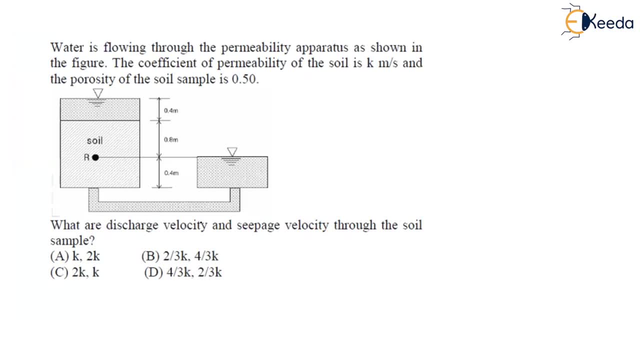 So, before finding the discharge velocity and seepage velocity, see, are these heads remains constant or are they changing? It seems like they are constant. right, They have maintained water level in such a way that these heads are not changing. Otherwise they should give some virtual diagram here, such that their water levels are decreasing and increasing. 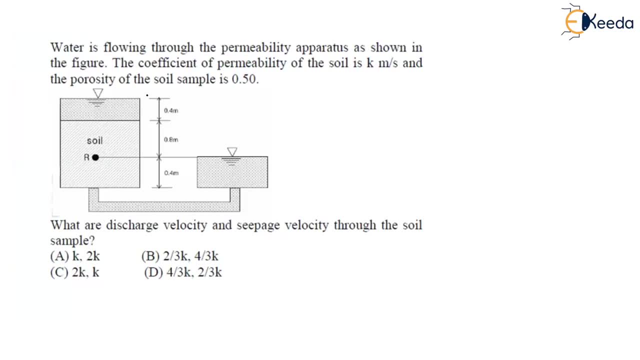 Then only we can understand that it is a variable head, As nothing is mentioned, so it is a constant head test. How we will find the discharge then? Discharge is nothing but Q equal to K into I into K, But here they are not interested in the discharge. 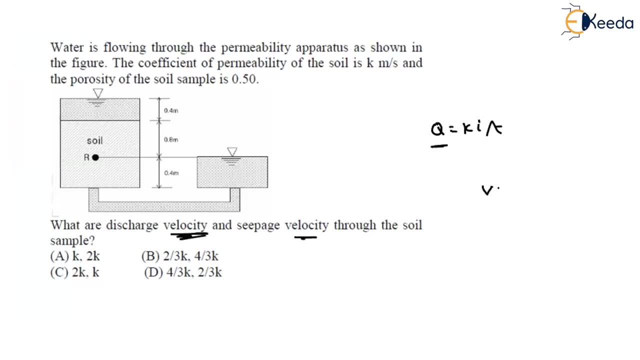 They are interested in the velocity. So how can I find the velocity? It is nothing but K into I. So this is what? nothing but your discharge velocity. Permeability itself is given K. Then what about the I value? I is nothing but a hydraulic gradient. 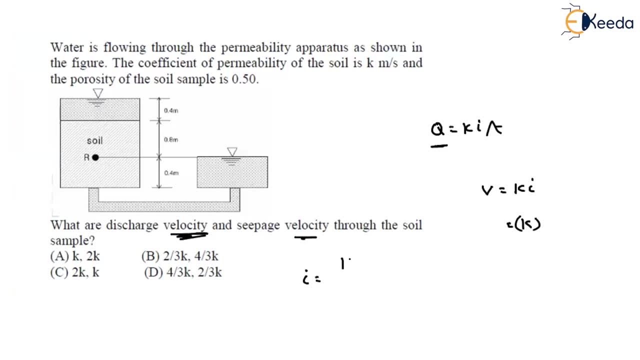 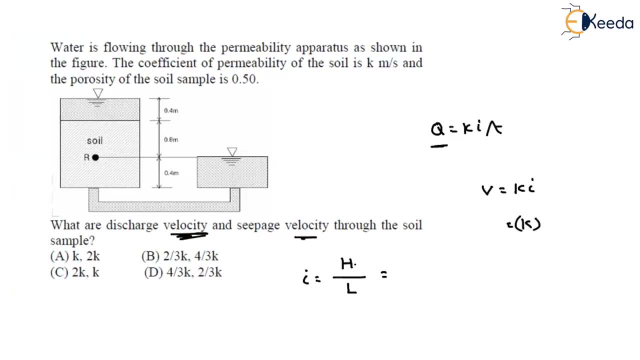 Always taken as a difference between the water level. So here it is the upstream water level, It is a downstream water level. So what is the difference between the water levels? 0.4 plus 0.8.. That is nothing but a 1.2.. 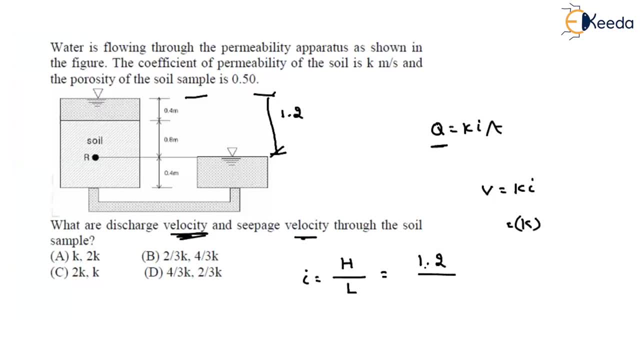 So the total head of the soil sample is nothing but a 1.2.. What is the length of the soil specimen from here to here? 0.8 plus 0.4.. Then again, it is how much 1.2.. 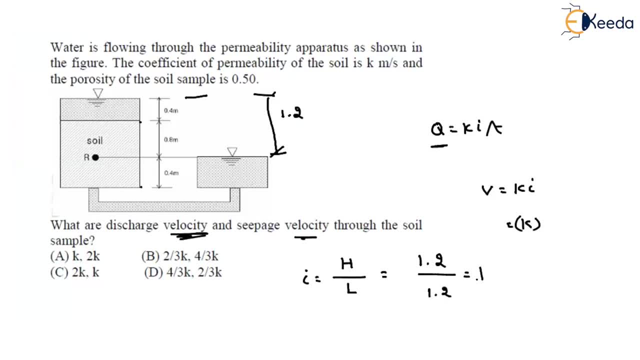 So for the present soil sample, what is the hydraulic gradient 1.. So if I substitute 1 here? so what is the discharge velocity? Discharge velocity is nothing but a K. How many options are there with K? Okay, there is only 1 K. 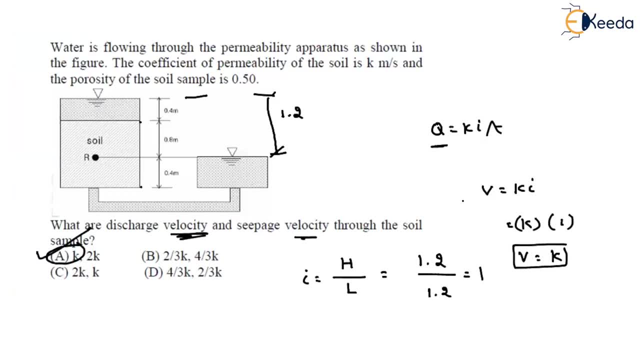 So directly you can choose this answer. Otherwise you can cross-check it by finding the seepage velocity. also, How can I find the seepage velocity? So let us say V, subscript S. So seepage. Seepage velocity is based on the force of the soil. 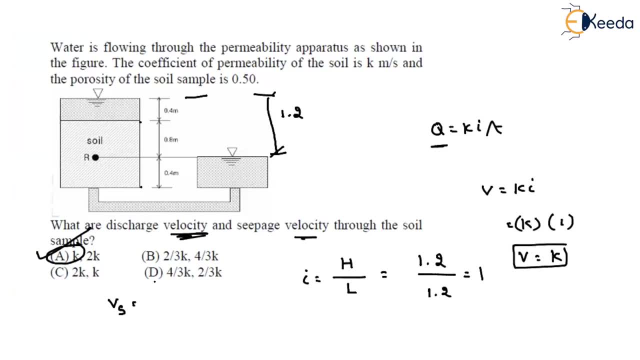 Discharge velocity is by considering the entire area of the soil. So seepage velocity is much more higher than the discharge velocity. How can I find it out? Just by discharge velocity divided by porosity. So discharge velocity is K.